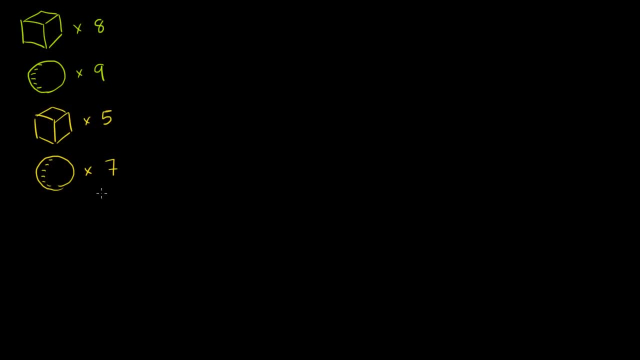 and then I'm going to pour it out and I'm going to look at the first object that falls out of that bag. What I want to think about in this video is: what are the probabilities of getting different types of objects? For example, what is the probability of getting a cube of any color? 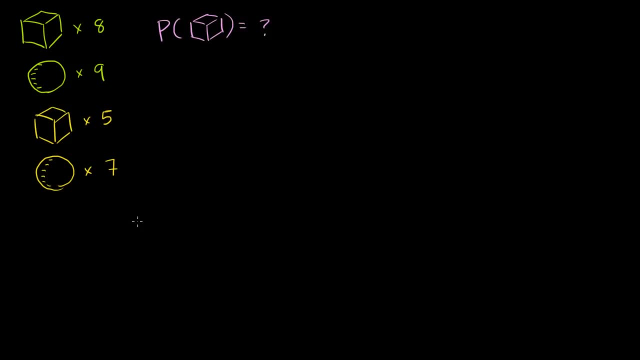 What is the probability? Well, to think about that we should think about, or this is one way to think about it- what are all of the equally likely possibilities that might pop out of the bag. Well, we have 8 plus 9 is 17.. 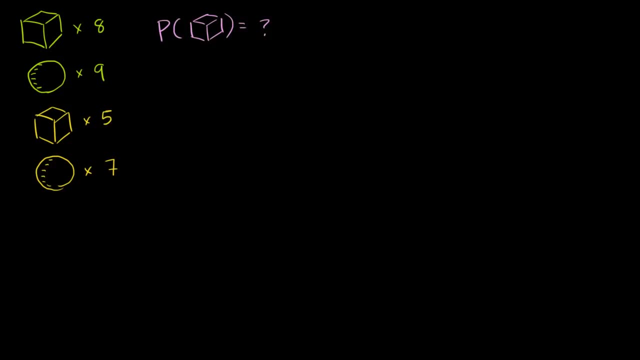 17 plus 5 is 22.. 22 plus 7 is 29.. So we have 29 objects. There are 29 objects in the bag. Did I do that right? This is 14.. Yep, 29 objects. 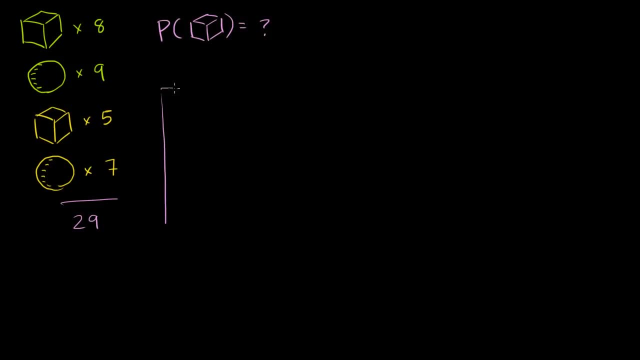 So let's draw all of the possible objects And I'll represent it as this big area right over here: 0. So these are all the possible objects. There are 29 possible objects, So there's 29 equal possibilities for the outcome of my experiment. 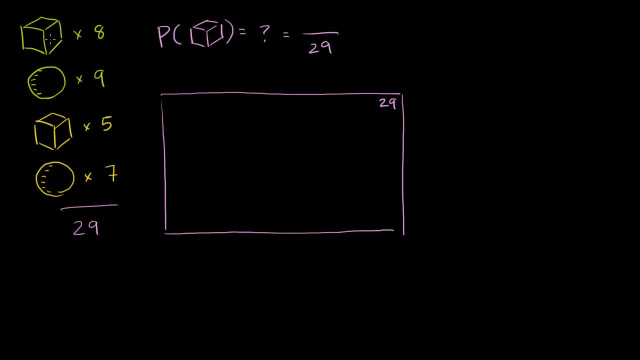 of seeing what pops out of that bag, assuming that it's equally likely for a cube or a sphere to pop out first, And how many of them meet our constraint of being a cube? Well, I have 8 green cubes and I have 5 yellow cubes. 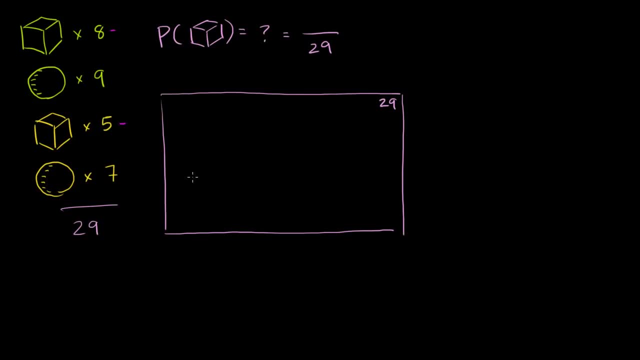 So there are a total of 13 cubes And so let me draw that set of cubes. So there's 13 cubes. I could draw it like that, Like this: There are 13 cubes. This right here is the set of cubes. 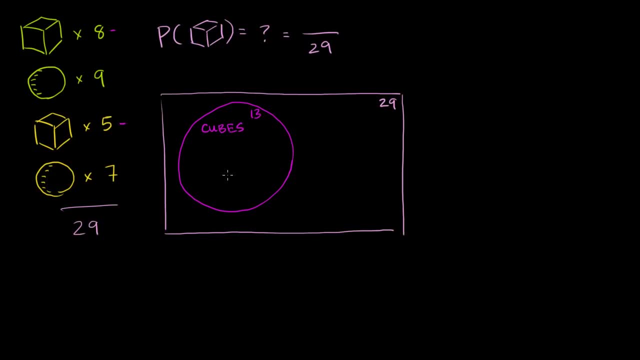 This area- and I'm not drawing it exact, I'm approximating- represents the set of all the cubes. So the probability of getting a cube is the number of events that meet our criterion. So there's 13 possible cubes that have an equal likely chance. 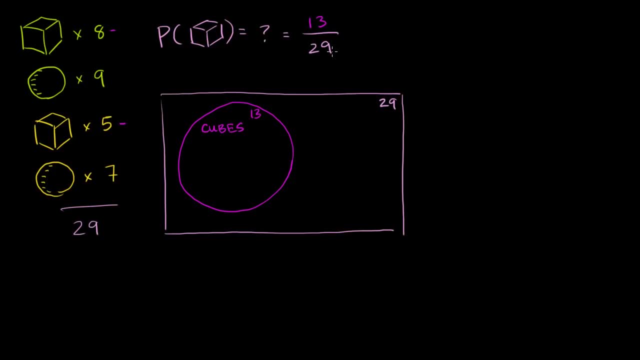 of popping out over all of the possible, equally likely events, which are 29.. That includes the cubes And the spheres. Now let's ask a different question: What is the probability of getting a yellow object, either a cube or a sphere? 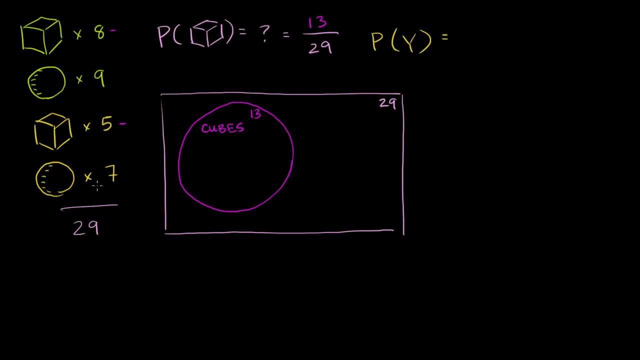 So, once again, how many things meet our conditions here? Well, we have 5 plus 7.. There's 12 yellow objects in the bag, So we have 29 equally likely possibilities. I'll do that in the same color. We have 29 equally likely possibilities. 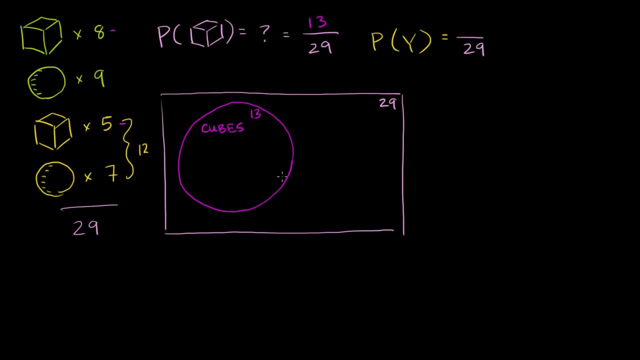 And of those 12 meet our criterion. So let's say let me draw 12 right over here, Let me do my best attempt. So let's say it looks something like. so the set of yellow objects: there are 12.. 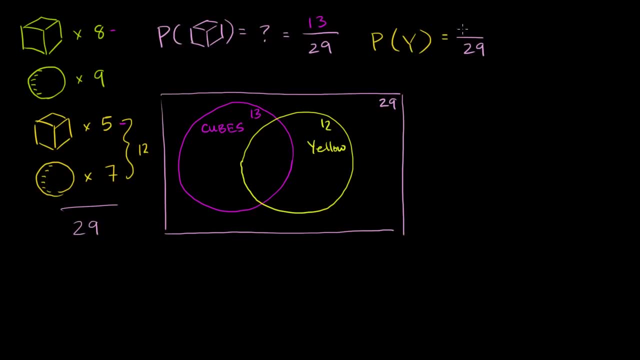 There are 12 objects that are yellow, So the 12 that meet our conditions are 12 over all the possibilities 29.. So the probability of getting a cube: 13- 29s. Probability of getting a yellow: 12- 29s. 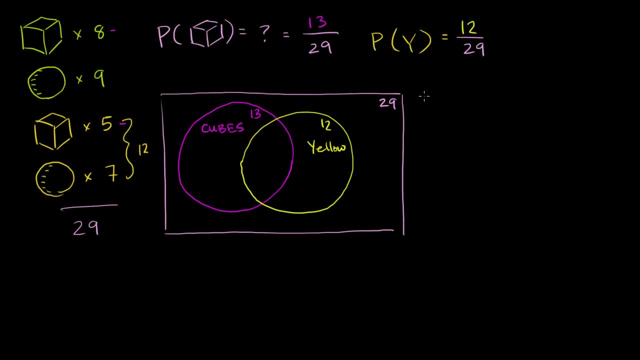 Now let's ask something A little bit more interesting. What is the probability? what is the probability of getting a yellow cube? So I'll put it in yellow, So we care about the color now. So this thing is yellow. What is the probability of? or, as my son would say, lello. 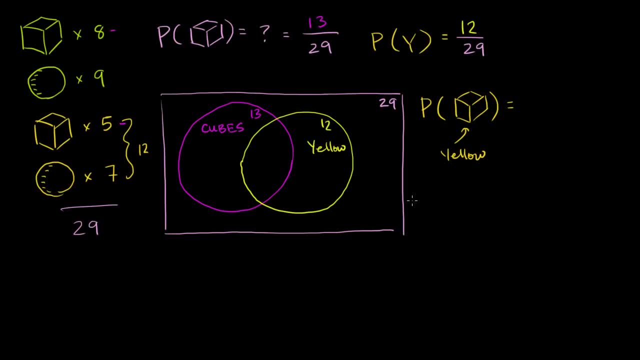 What is the probability of getting a yellow cube? Well, there's 29 equally likely possibilities. There's 29 equally likely possibilities, And of those 29 equally likely possibilities, five of those are yellow cubes Or lello cubes. five of them. 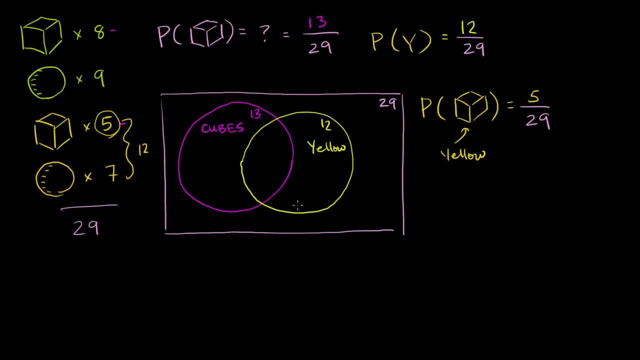 So the probability is five, 29s, And where would we see that? on this Venn diagram that I have drawn. And this Venn diagram. this is just a way to visualize the different probabilities And they become interesting when you start thinking about. 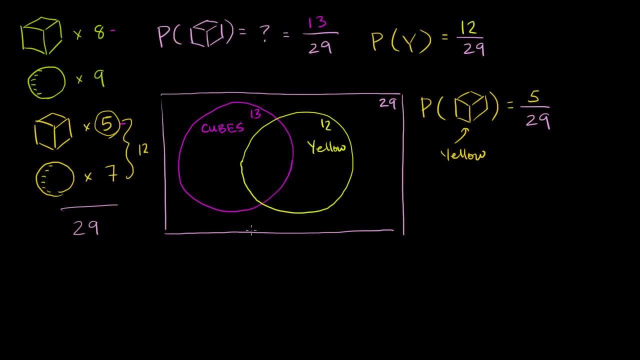 where sets overlap or even where they don't overlap. So here we're thinking about things that are members of the set yellow, so they're in this set and they are cubes, So this area right over here, that's the overlap of these two sets. 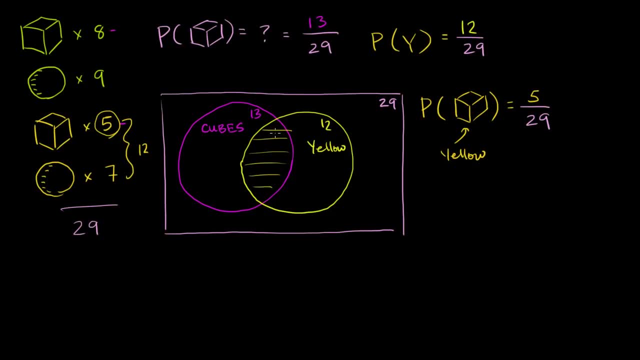 So this area right over here, this represents things that are both yellow and cubes, because they are inside both circles. So this right over here, let me write it over here: So there's five objects that are both yellow and cubes. Now let's ask, and this is probably the most interesting: 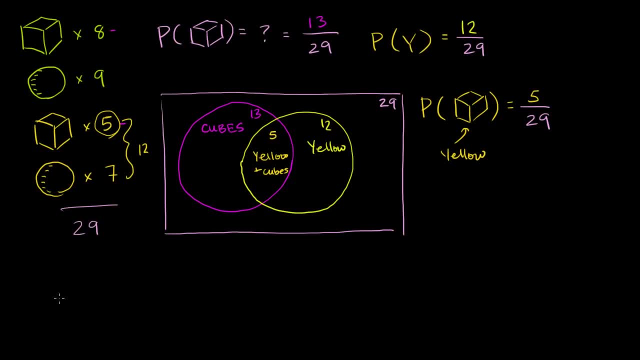 thing to ask: what is the probability of getting something that is yellow or a cube, a cube of any color? Probability of getting something that is yellow or a cube of any color. Well, we still know that the denominator here is going to be 29.. 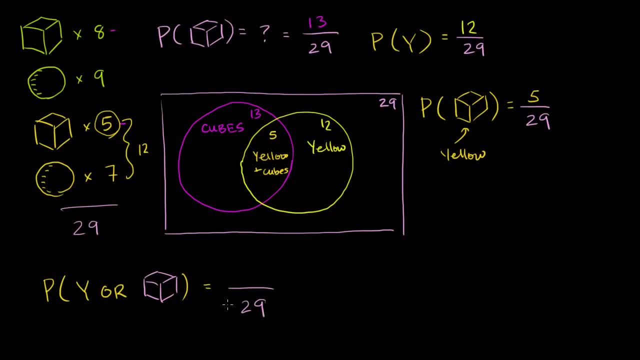 These are all of the equally likely possibilities that might jump out of the bag. But what are the possibilities that meet our conditions? Well, one way to think about it, one way to think about it is: well, there's 12 things that would meet. 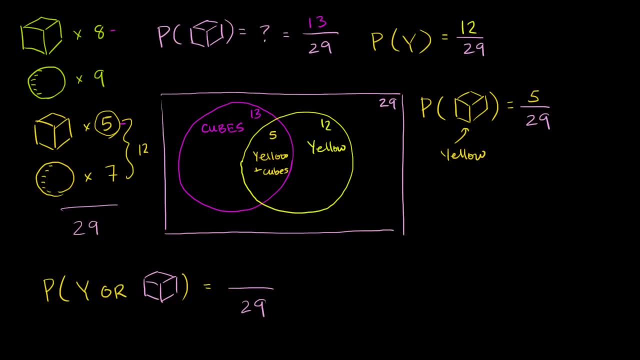 the yellow condition. So there's 12 things that would meet the yellow condition. So there's 12 things that would meet the yellow condition. So that would be this entire circle right over here: 12 things that meet the yellow condition. So this right over here is 12.. 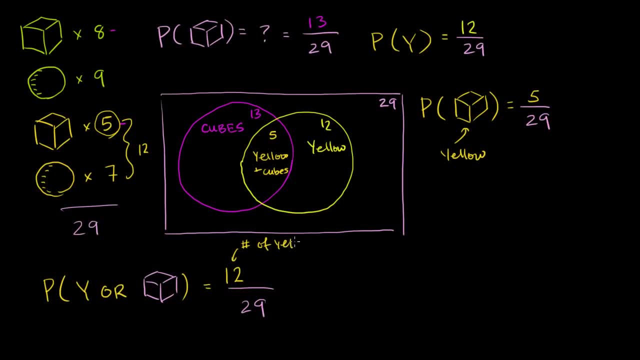 This is the number of yellow, That is 12.. And then to that we can't just add the number of cubes, because if we add the number of cubes we've already counted these five. These five are counted as part of this 12.. 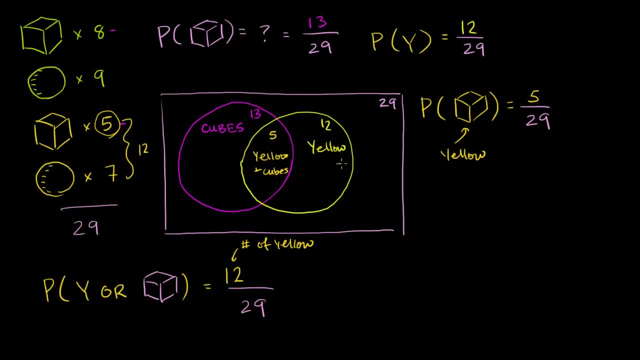 One way to think about it is: there are seven yellow objects that are not cubes. Those are the spheres. There are five yellow objects that are cubes, And then there are eight cubes that are not yellow. That's one way to think about it. 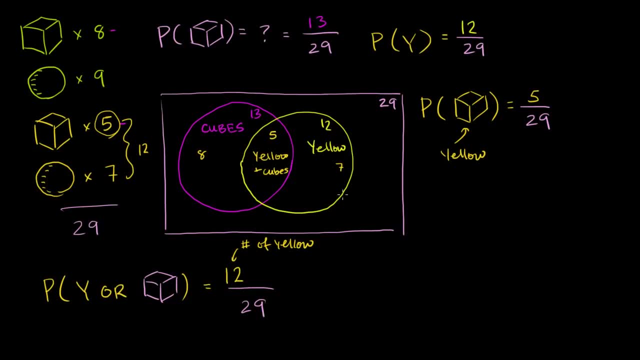 So when we counted this 12, the number of yellow, we counted all of this. So we can't just add the number of cubes to it, because then we would count this middle part again. So then we have to essentially count cubes. 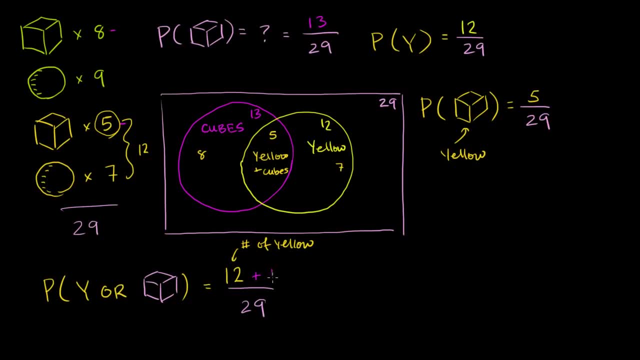 the number of cubes, which is 13.. 13. So the number of cubes, Number of cubes, Number of cubes. And we'll have to subtract out this middle section right here, Right over here, Let me do this. So subtract out the middle section right over here. 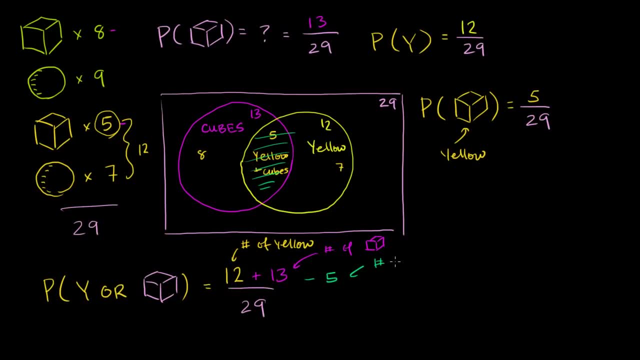 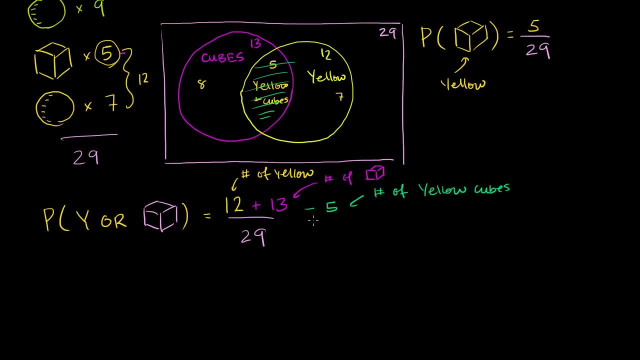 So minus 5.. So this is the number of yellow cubes. It feels weird to write the word yellow in green- The number of yellow cubes, Or another way to think about it, and you could just do this math right here: 12 plus 13 minus 5 is what. 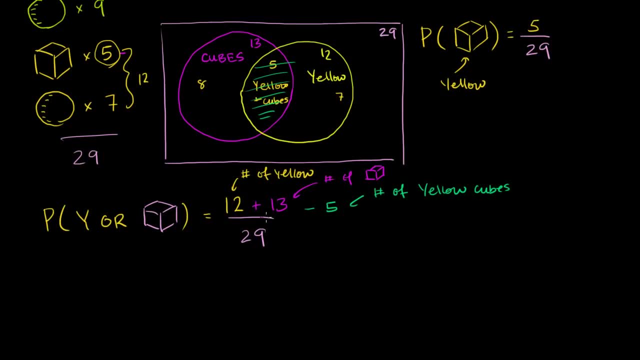 It's 20.. Did I do that right? 12 minus yep, it's 20.. So that's one way You would just get. this is equal to 20 over 29.. But the more interesting thing than even the answer: 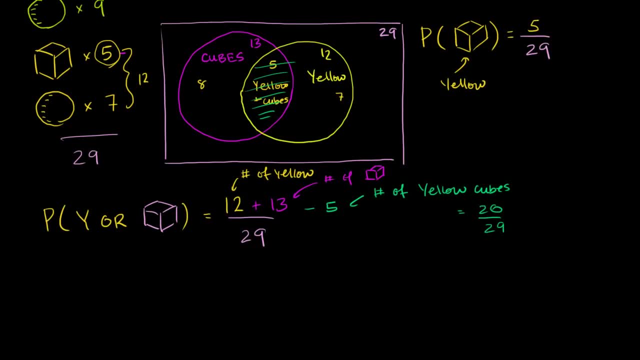 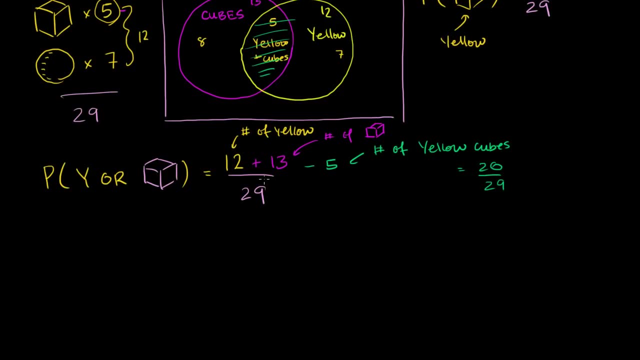 of the probability of getting. that is expressing this in terms of the other probabilities that we figured out earlier in the video. So let's think about this a little bit. We can rewrite this fraction right over here. We can rewrite this as 12 over 29. 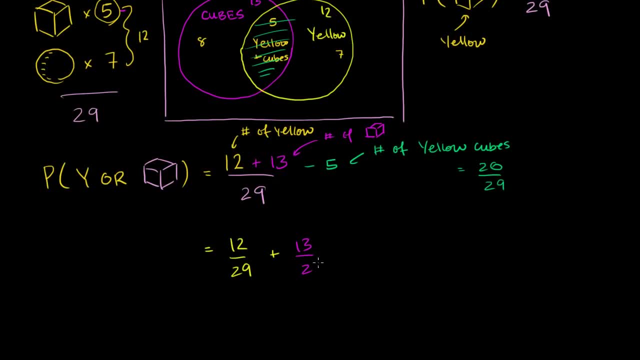 plus 13 over 29, minus 5 over 29.. Minus 5 over 29.. And this was the number of yellow over the total possibilities. So this right over here was the probability of getting a yellow. This right over here was the number of cubes over the total possibilities. 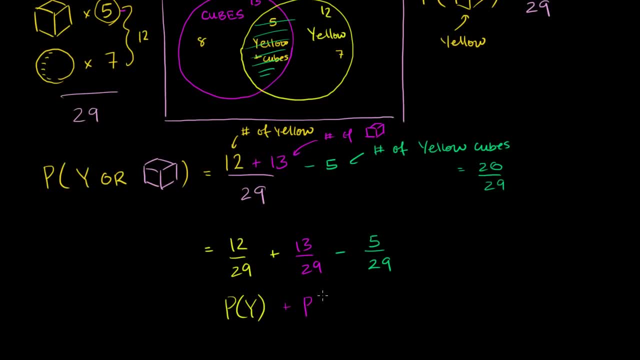 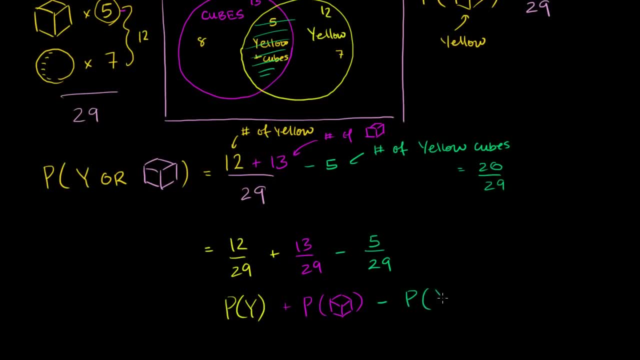 So this right over here was minus the probability of yellow over the total possibilities. So this right over here was minus the probability of yellow and a cube, And let me write it that way- Minus the probability of yellow. I'll write yellow in yellow. 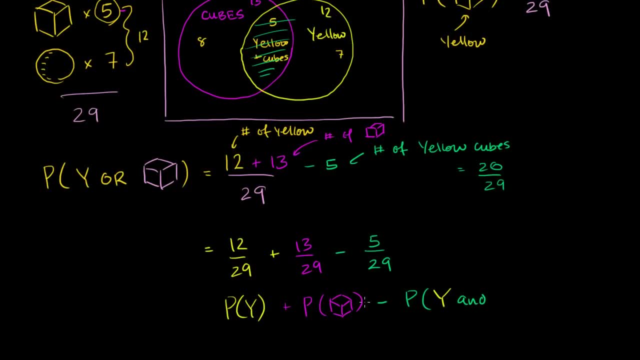 Yellow and getting a cube, And so what we've just done here, and you could play with the numbers- The numbers I just used as an example right here to make things a little bit concrete. But you can see this is a generalizable thing. 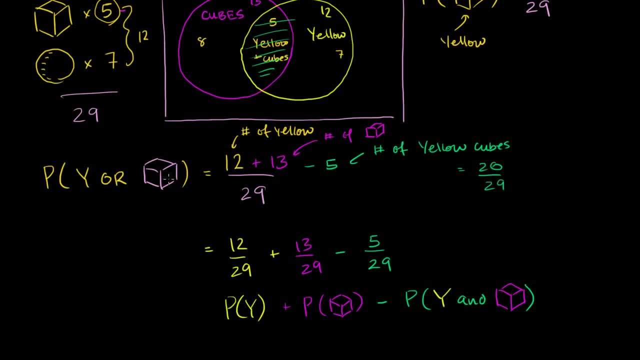 If we're going to get a cube, If we're going to get a cube, If we're going to get a cube, If we have the probability of one condition or another condition. So let me rewrite it, The probability, And I'll just write it a little bit more generally here. 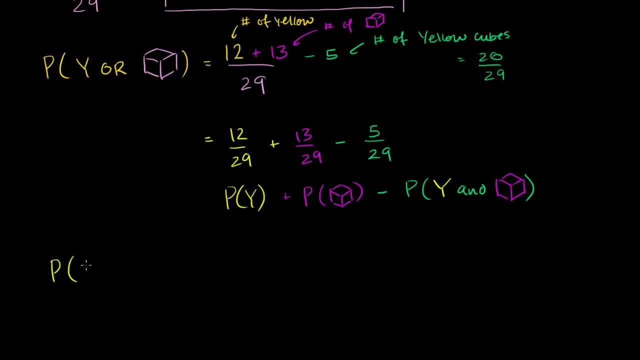 This gives us an interesting idea. The probability of getting one condition Of an object being a member of set A or a member of set B Is equal to the probability that it is a member of set A Plus the probability that it is a member of set B. 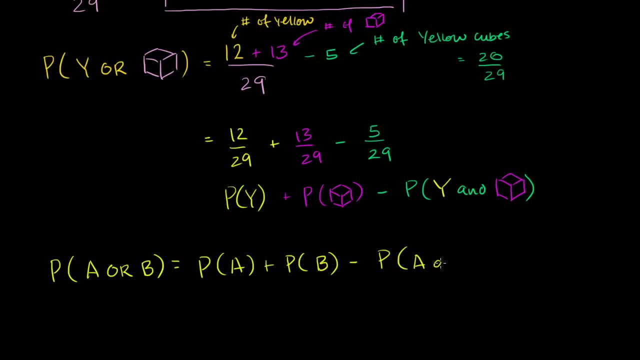 Minus the probability that it is a member of both, Minus the probability that it is a member of both, Minus the probability that it is a member of both, And this is a really useful result, I think. sometimes it's called like the addition rule of probability. 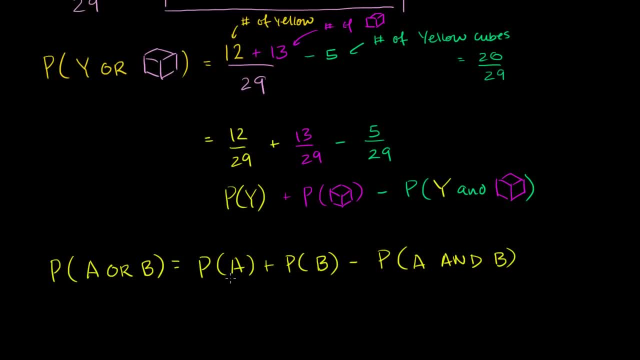 But I wanted to show you it's a completely common sense thing. The reason why you can't just add these two probabilities Is because they might have some overlap. There's a probability of getting both, And if you just added both of these,